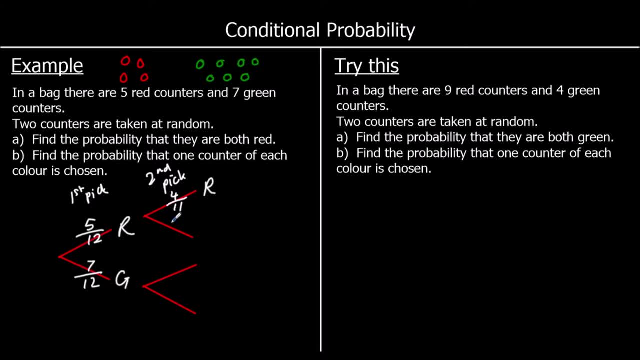 and the chance of getting a green is seven out of eleven. Let's go back to the start. If we picked out a green to start with- so we picked out a green- a green's gone. the chance of getting a red would be five out of eleven. 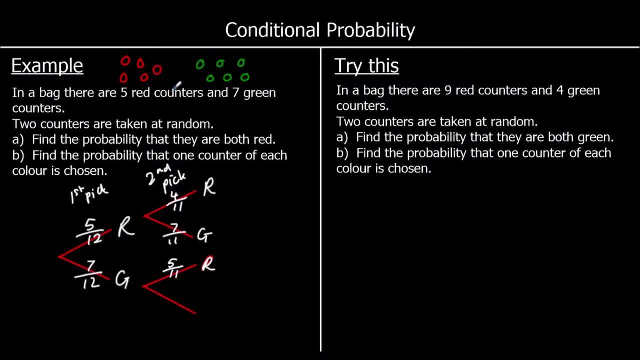 and the chance of getting a green. there are six left out of eleven, So they are all our probabilities. Now let's look for the probability that they're both red, So it's five. twelfths. When we go across the branch we're going to have times. So for red, red. 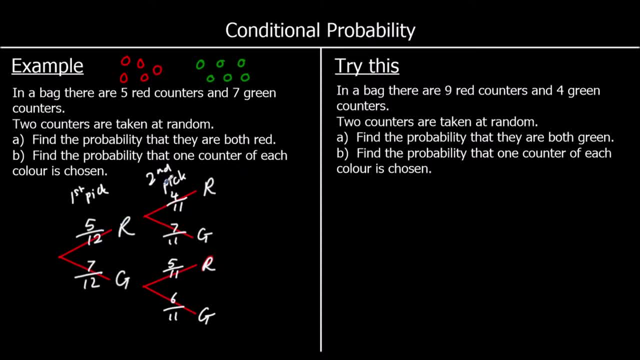 it's going to be five twelfths times four elevenths, So the chance of getting two reds is five times four over twelve times eleven. So twenty out of a hundred and thirty-two The chance of getting a red, then a green. 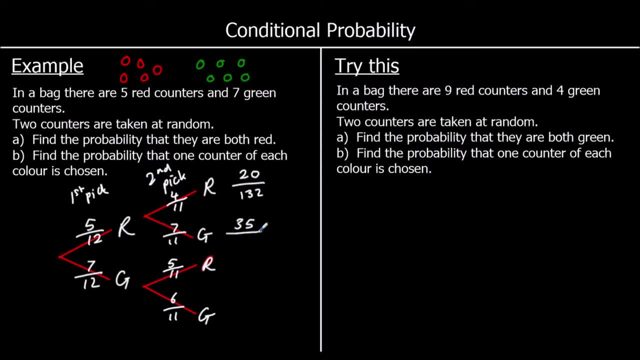 is going to be five times seven, which is thirty-five out of a hundred and thirty-two. Green and red, seven times five, thirty-five out of a hundred and thirty-two, and green and green is going to be seven sixths, which is forty-two out of a hundred and thirty-two. 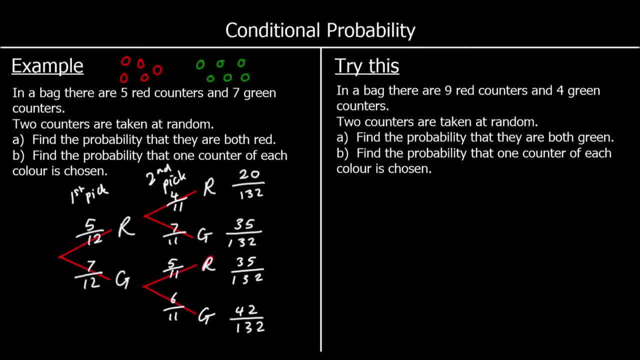 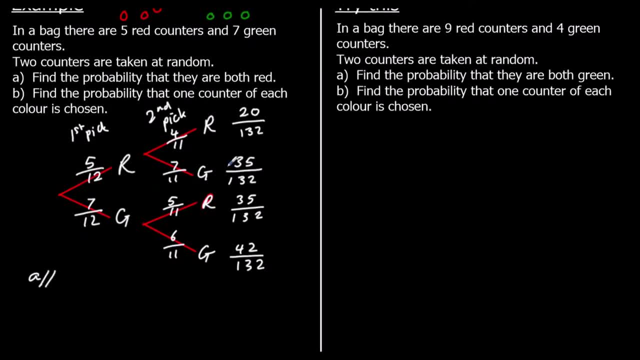 So they are all our probabilities. So, to answer part A, the probability that they're both red is twenty out of a hundred and thirty-two. We don't have to simplify it unless we're asked to, so I'm going to leave it. So I'm going to leave it. 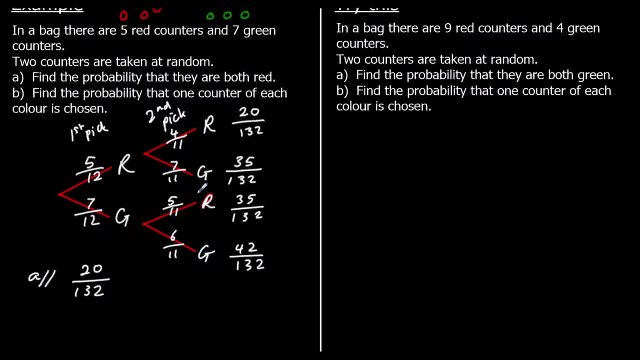 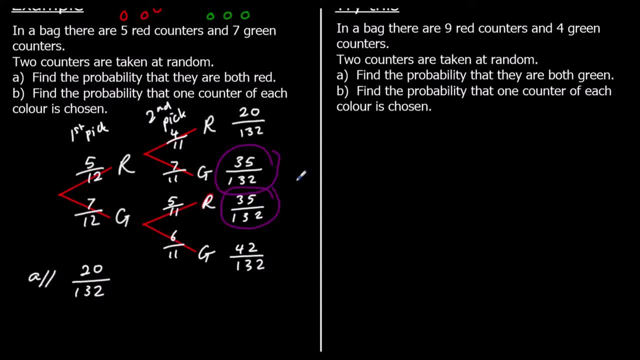 so red green or green red, so thirty-five and thirty-five, so there's seventy in total. So for B, seventy out of a hundred and thirty-two, And you'll notice that all of these probabilities add up. they're all the options. 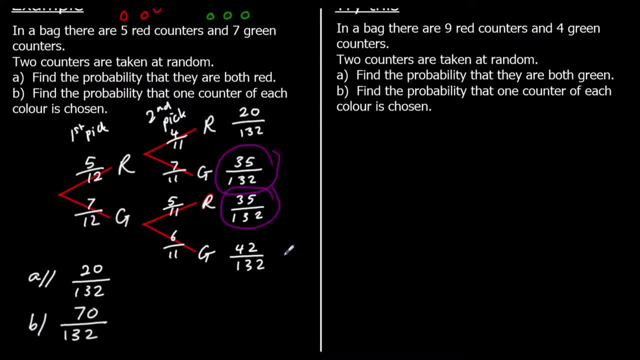 all the possible options add up to a hundred and thirty-two. out of a hundred and thirty-two, We can either get red, red, red green, green red or green green. there's no other option, so those probabilities have to add up to a whole. 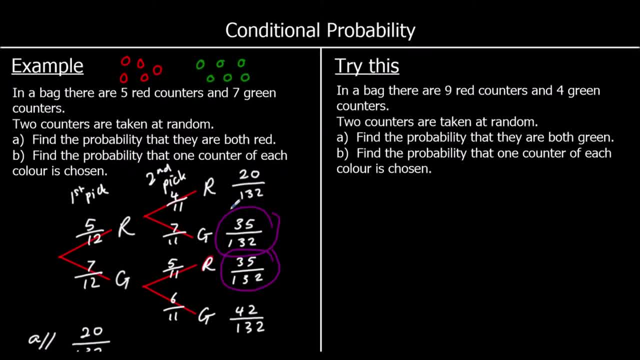 Okay, one for you to try, so give this one a go. So this time we've got nine red and four green, but apart from that, it's the same as the last question, So we can get red, green, red, green, red or green. 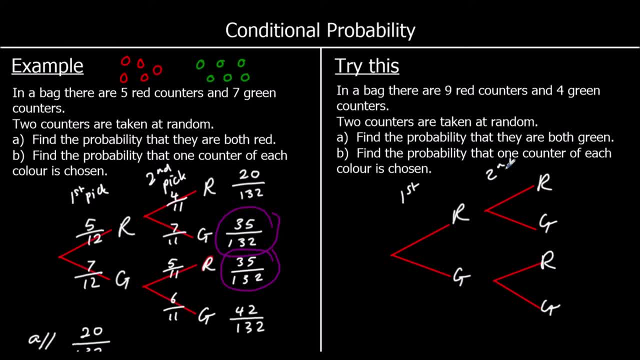 So the first counter and the second counter. So for the first counter, there were nine red out of thirteen in total and four green out of thirteen in total. If we took a red- if we took a red- there'd only be eight reds left out of twelve in total. 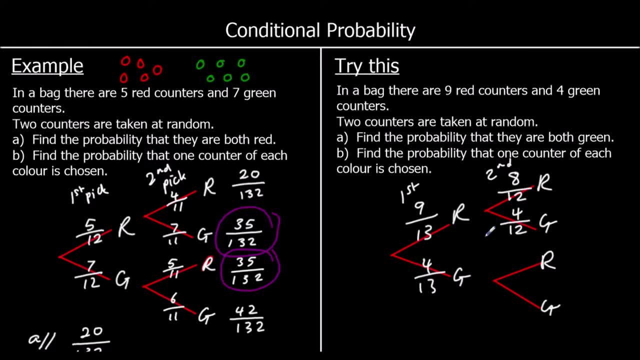 and all the greens would still be there. so four out of twelve because one red's gone, And if we took a green first, there'd only be three greens left out of twelve and nine red left out of twelve. So the probabilities, I'll work them all out. 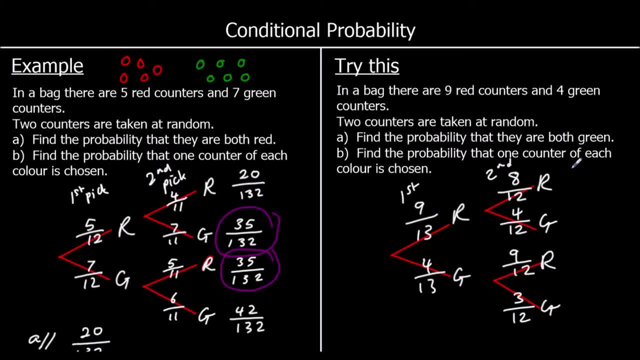 So red, then red. nine times eight is seventy-two. Thirteen times twelve. well, twelve twelves are a hundred and forty-four plus another twelve, so a hundred and fifty-six. Nine thirteenths times four, twelfths will be thirty-six. 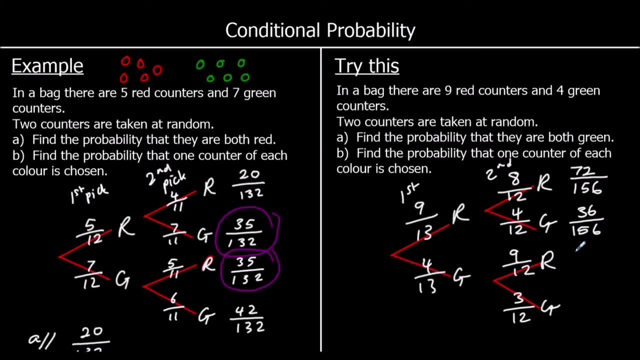 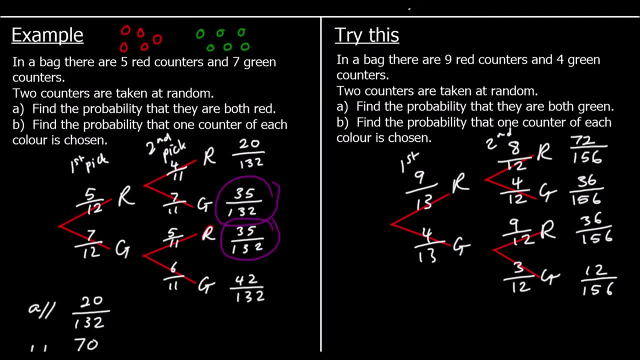 Out of a hundred and fifty-six. Four, nines, thirty-six Out of a hundred and fifty-six, And four, threes are twelve And again that'll be out of a hundred and fifty-six. So what were the questions? Part A: find the probability. they're both green. 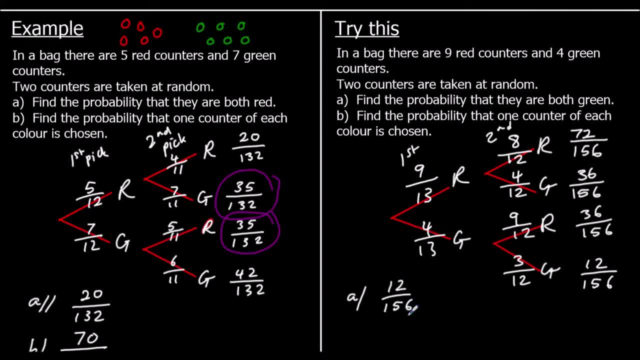 Twelve out of a hundred and fifty-six. We don't have to simplify our answer. we could, but unless we're asked to we don't have to do it. And for part B, one of each colour say thirty-six and thirty-six, that's going to be seventy-two. 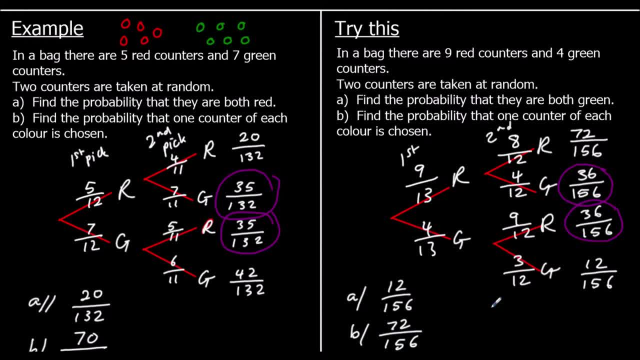 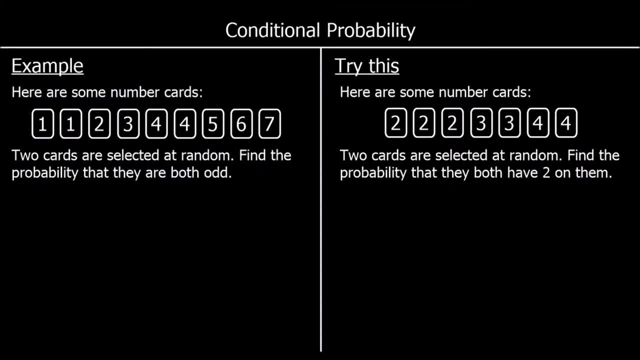 So seventy-two out of a hundred and fifty-six. Here's another question. this time we've got number cards and the question says two cards are selected at random. find the probability. they're both odd. So again we could draw a tree diagram. 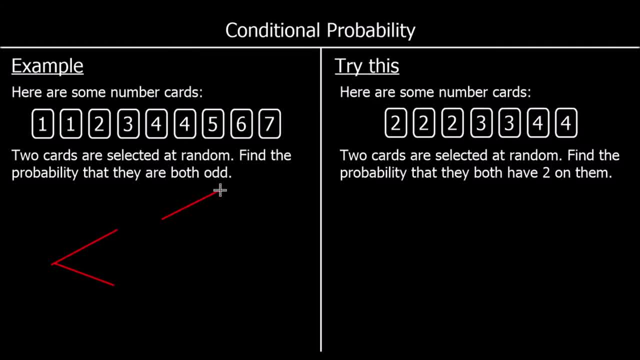 We can have even and odd or odd and even either way round. So it's our first card and our second card Let's go with odd, even, odd, even odd. even So, there are one, two, three, four, five odd. 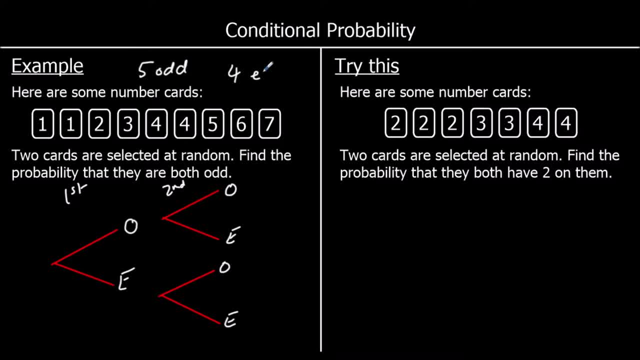 And one, two, three, four, even So there's nine in total. Five are odd and four are, even So the probability of getting an odd the first time is five out of nine. Five out of nine are odd and the first time the probability of getting even. 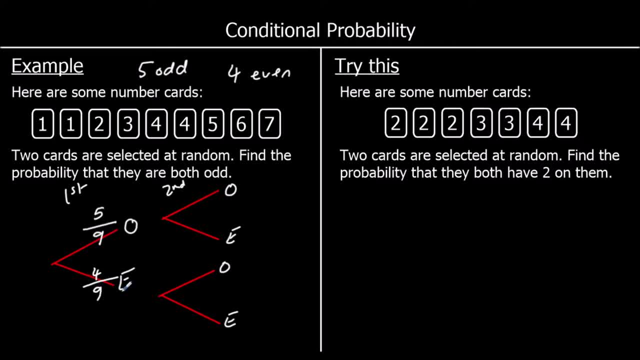 is four ninths. Now, if we remove an odd, if we take an odd out, there'll be four odds out of eight left and four evens out of eight, And if we take an even out, there'll be three evens left out of eight. 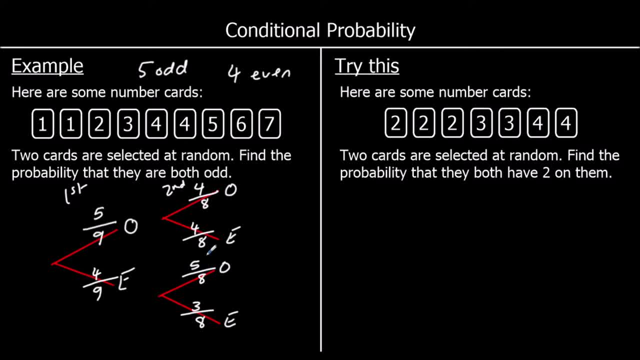 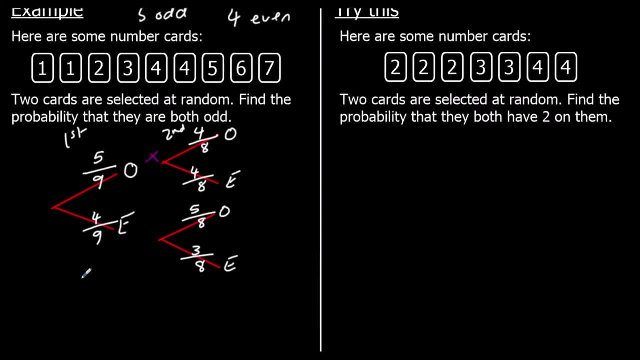 and five odds left out of eight. So the question was the probability of getting two odds. so it's going to be five ninths times four eighths, which is 20 out of 72. We could simplify it. we could have five eighteenths. 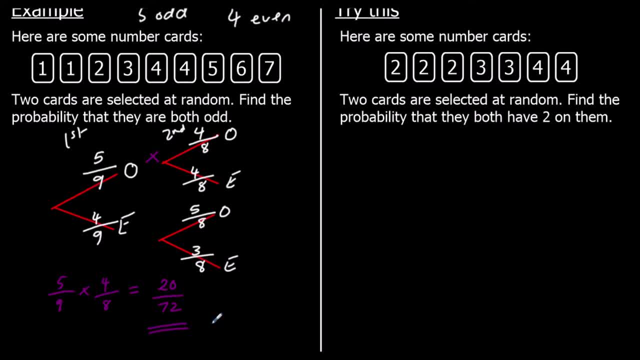 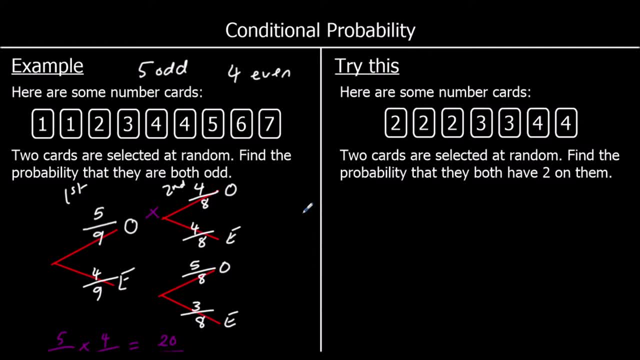 but we don't have to, so we can leave it like that, And here's one for you to try, So give this one a go. So this time we want to know the probability that two cards again, two cards are getting picked again. 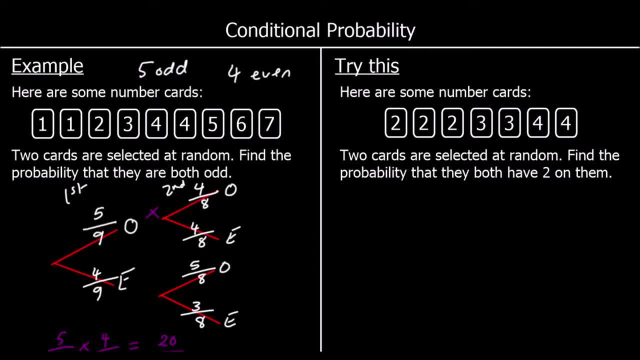 the probability they both have a two on them. So we could draw a tree diagram again or we could skip. we could skip drawing the tree diagram. We could draw a tree diagram of two and not two, or we could say the probability of getting a two the first time is three sevenths. 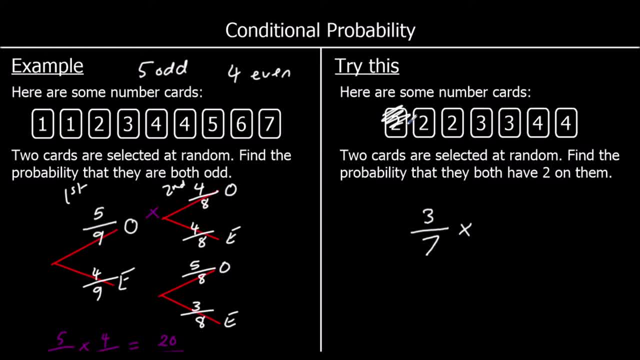 and for the second time, if we remove the two, we've got two twos left out of six. So it's going to be: if we did draw a tree diagram, the calculation we'd end up with is three sevenths times two sixths. 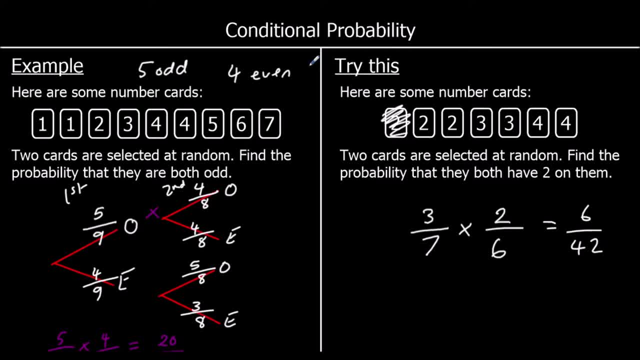 which is six over 42. We don't have to simplify that. we can leave it as six over 42.. We can leave it as six over 42. We don't have to simplify that. we can leave it as six over 42.. 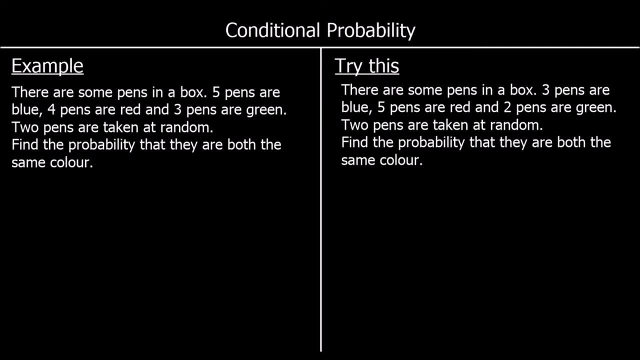 And another example. this time we have three different things. So we've got pens in a box. five pens are blue, four pens are red and three pens are green. So if we're drawing a tree diagram, we're going to have three different options. 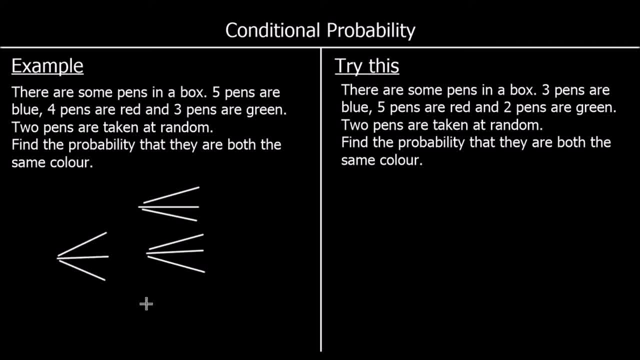 three different parts to each of our branches. So it's going to look something like that: And we've got blue, red and green. So we've got five blue pens, four red pens and three green pens, So we can have blue red. 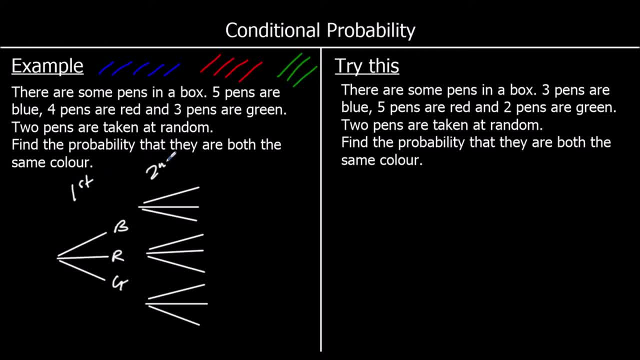 and green for the first pen and the second pen, Blue, red green. blue, red green, blue, red green. For the first pen, the chance of getting a blue is five out of twelve. five out of twelve. 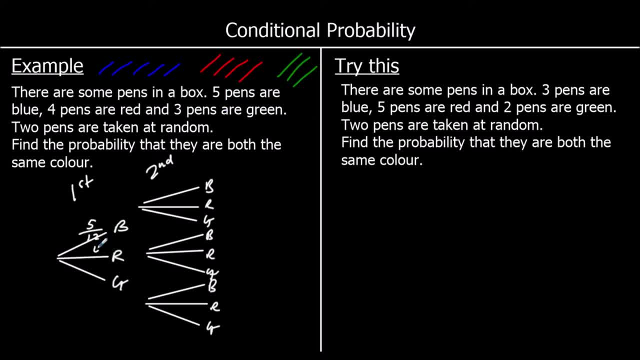 The chance of getting a red is four twelfths and a green three twelfths For the second pen, if we took a blue pen out, if we got rid of a blue pen, there'll be four blue pens left out of eleven. 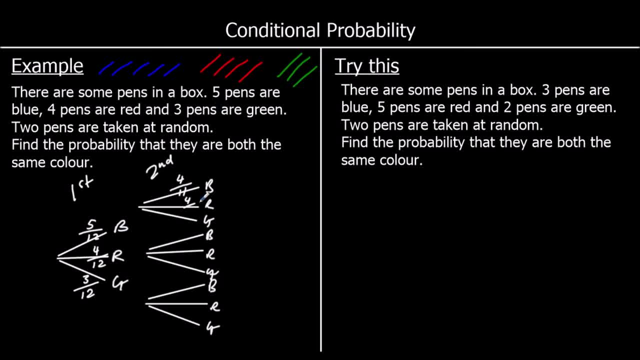 There'll be four red left out of eleven and three greens. If we took a red pen out, there'll be five blues out of eleven. There'll be three reds because we took one out And three greens. If we took a green pen out, there'll be five elevenths blue. 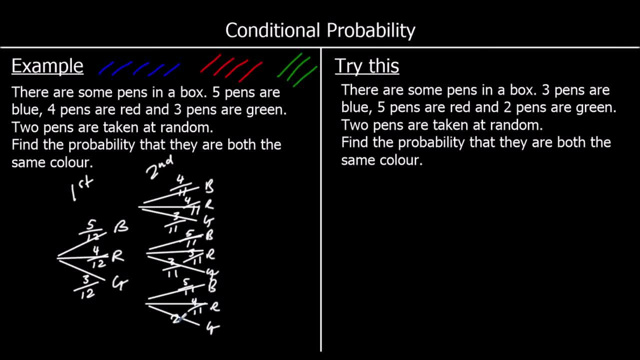 four elevenths red and two elevenths green, So the probability that both pens are the same colour. So for blue it's five twelfths times four elevenths five. fours are twenty twelve. elevens are a hundred and thirty-two. 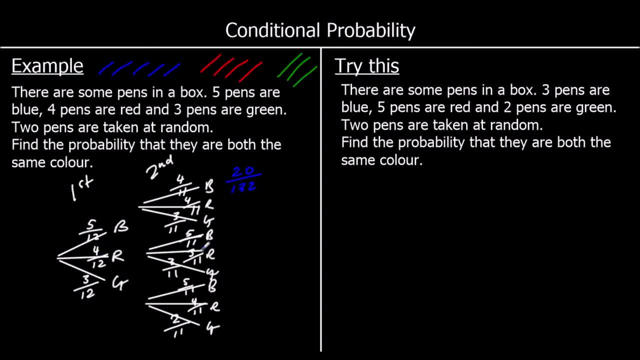 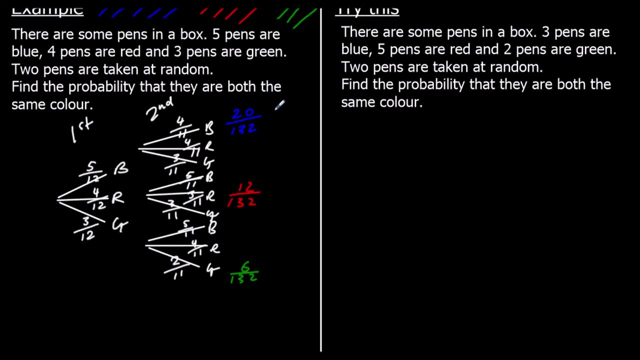 For red red, then red four times three is twelve and twelve elevenths is a hundred and thirty two, And for green: three, twos are six, twelve elevenths are a hundred and thirty two. So we've got twenty plus twelve plus six. 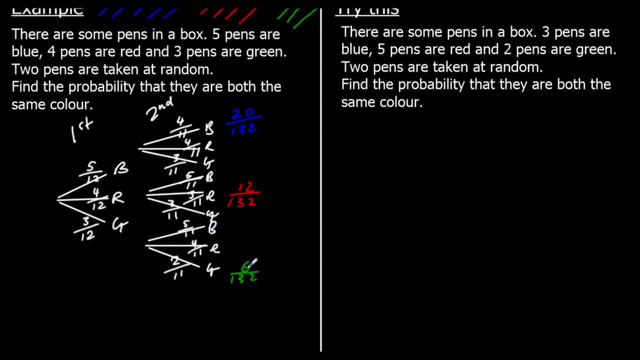 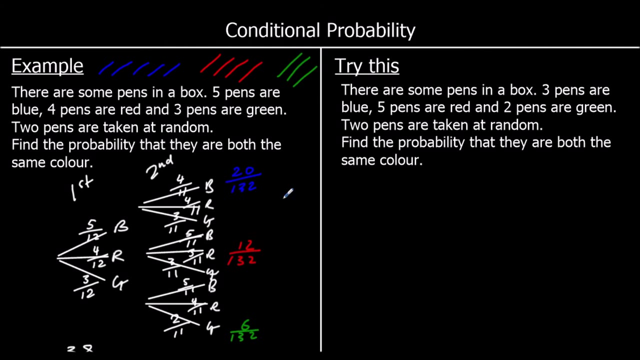 so that's twenty plus twelve plus six is 32 plus 6 makes 38. so 38 out of 132. again, I'm not gonna simplify unless I'm asked to, so I'm gonna leave it one for you to try. so give this one a go. so 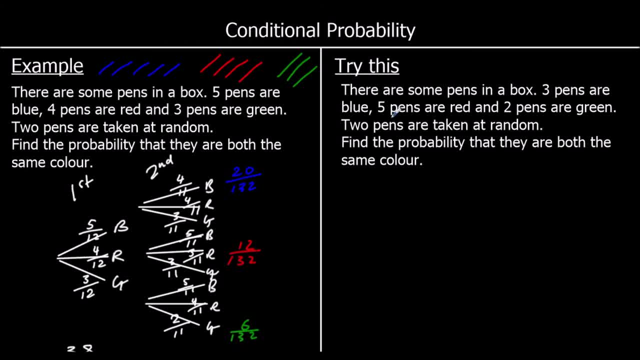 we've got some pens in a box: 3 blue, 5 red and 2 green. 2 pens are taken at random. again, find the probability that they're both the same color, so I'm not going to draw the tree diagram. if you did draw the tree diagram, you'll get the. 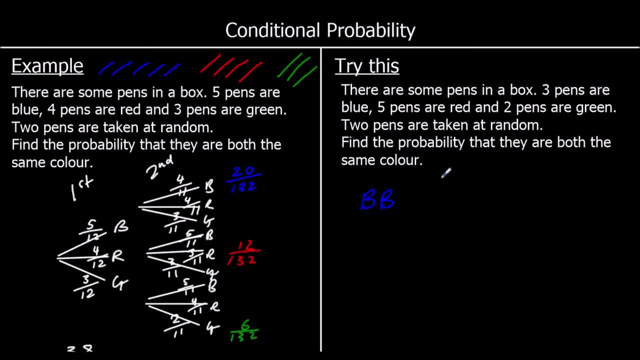 probability of blue. blue as 3 out of 10 times 2 out of 9 say 6, 90 of s. for red, then red it'll be 5 out of 10 times four 9, which is 20, 90 of s, and for 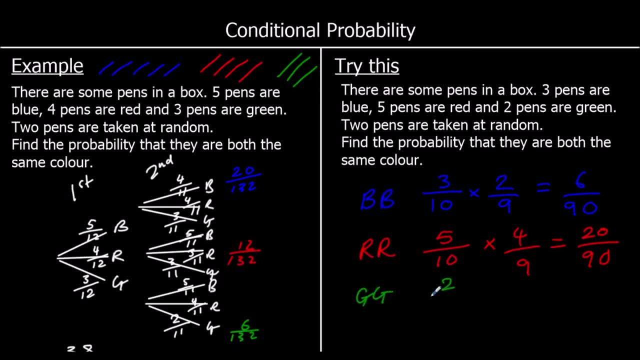 green, then green. 2 out of 10 times 1 out of 9, which is 2, nine tears to the probability of getting two pens the same color is 6, 90 of s, plus 20, ninety of s. for red, then red, it'll be 5 out of 10 times 4, nine, which is 20, ninety of s. and 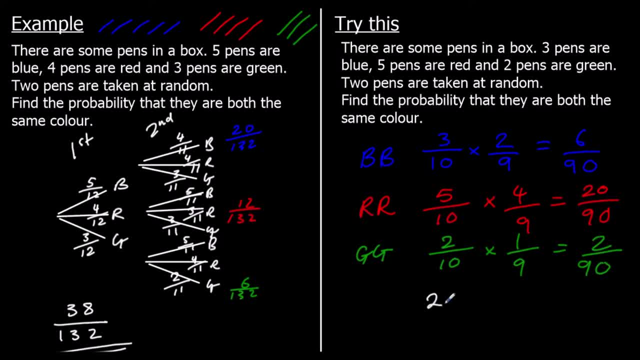 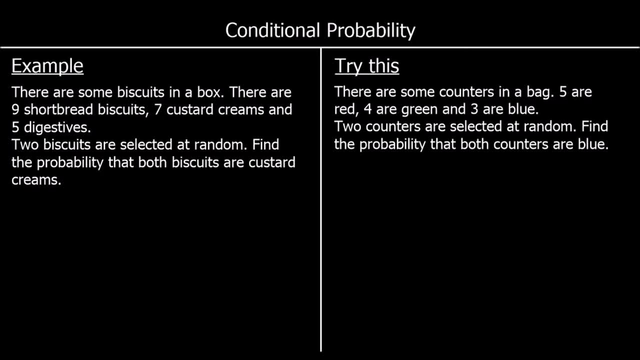 plus 2, 90 F's, which is 28: 90 F's. and another example: we've got biscuits in a box: 9 short red biscuits, 7 custard creams and 5 digestives. again, we're selecting 2 biscuits at random. find the probability that both biscuits are. 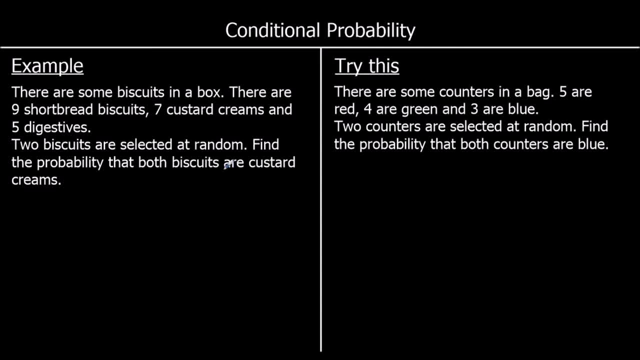 custard creams. so we only want to know the probability that they're both custard creams. so if we did, we could draw the tree diagram. it had three parts to it, but we only want custard creams. so what's the probability in the first biscuit being a custard cream? well, there are seven custard creams out of 9 plus. 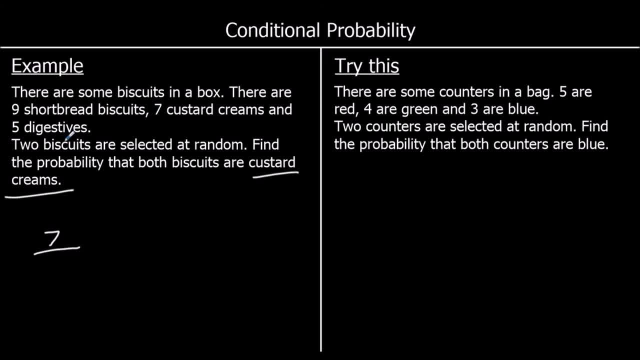 7 is 16 plus 5 is a custard cream. so we only want to know the probability that they're both custard creams. out of 9 plus 5 is 21, so 7 out of 21 for the first biscuit and then the second biscuit. if we took a custard cream out, there's 6. 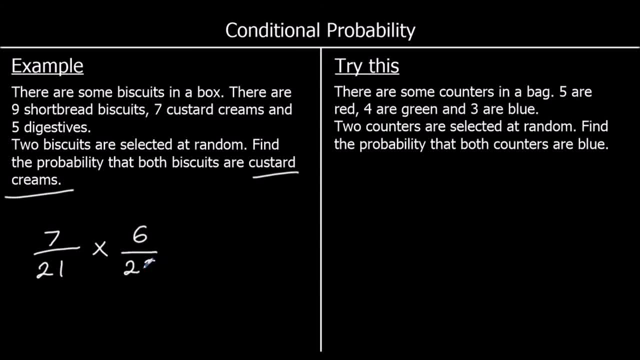 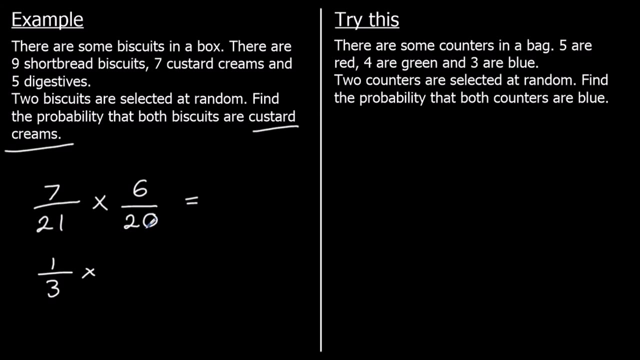 custard creams left out of 20 in total. so we're going to do 7 over 21 times 6 over 20. we could simplify this, which will actually make it a lot easier, but we'll do both. so 7 out of 21 is the same as a third. 6 out of 20 is the same as. 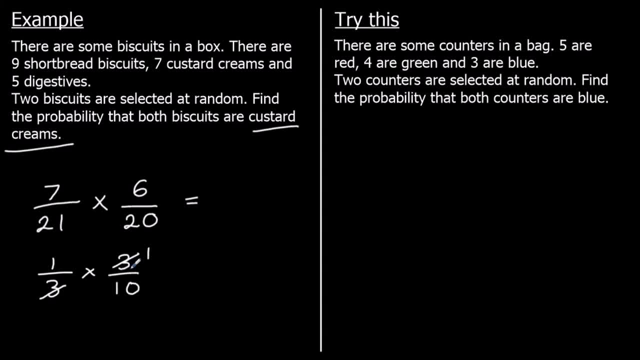 3 temps and we can even cancel these threes and say we've got one temp fear. so the answer is going to be one temp, simplified. if we didn't simplify it, we do 7 times 6, which is 42. over 21 times 6 is a third. so over 21 times 6 is a third. 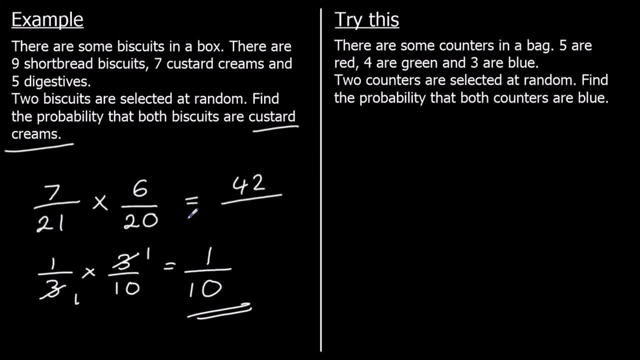 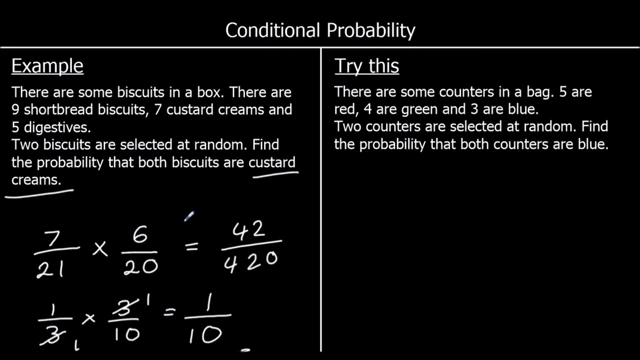 times 20, 20 20s are 400, plus another 20,, 420.. Either one of those two answers would be correct. they're both the same, they're equivalent. And one for you to try. so some counters in a bag- 5 red, 4 green, 3 blue, 2 are taken at random. find the probability. 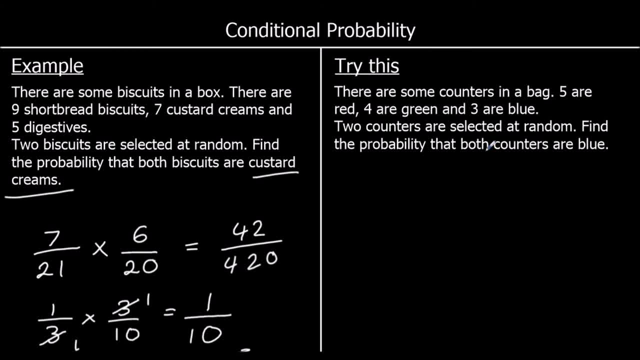 they're both blue. So for the first one to be blue, it'll be 3 out of 12, and if I took a blue one out, there'll be 2 blue left out of 11.. So 3 times 2 is 6,. 3 times 2 is 6,. 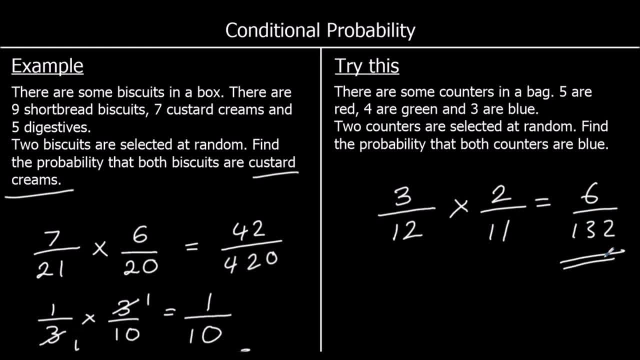 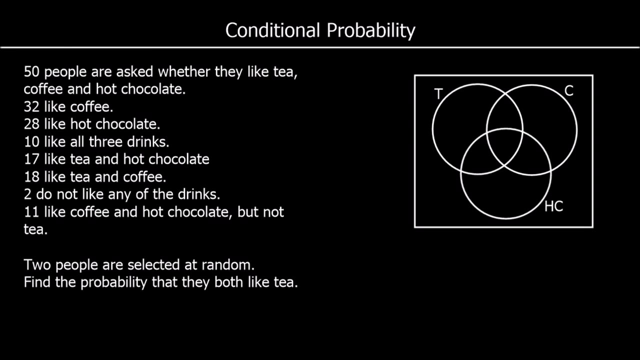 12 times 11 is 132, so we've got 6 out of 132.. And we could simplify that it would be 1 over 22,, but we don't have to do that. And one more question: this time we've got. 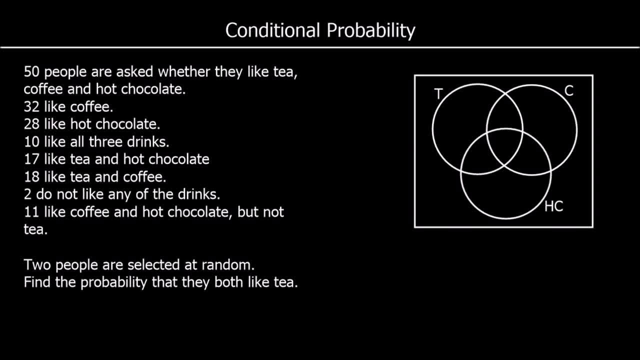 a Venn diagram to complete first. So if you want to pause the video and give it a go, try and do that, otherwise just keep watching. So we've got 50 people asked whether they like tea, coffee and hot chocolate. 32 like. 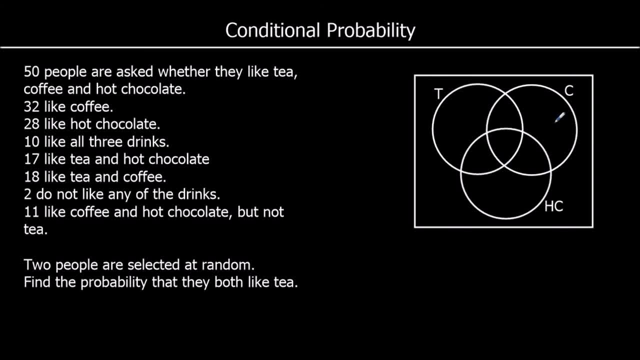 coffee. so that means the whole coffee circle is 32, so we can't do anything with that. at the moment it's 50 people in total: 32 like coffee, 28 like hot chocolate. we can't do anything with that information yet. 10 like all 3 drinks. 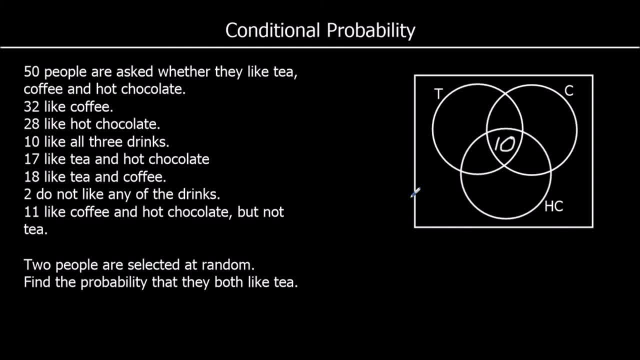 So we like to start in the middle of the Venn diagram and work out: 10 like all 3 drinks, 17 like tea and hot chocolate. so tea and hot chocolate, the overlap of them must be 17,. we've already got 10, so we need 7 more. 18 like tea and coffee. so the overlap between 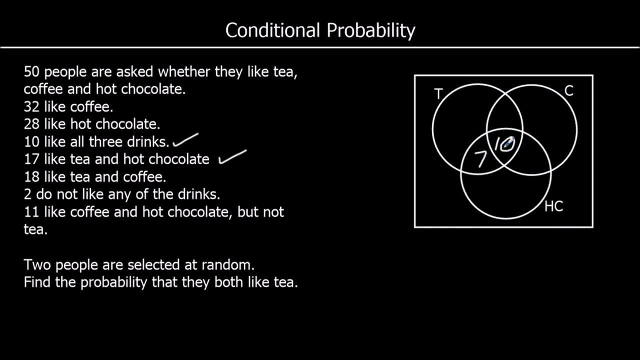 tea and coffee must be 18,. we've already got 10, so we need 8 more. 2: do not like any of the drinks so they go on the outside. 11: like coffee and hot chocolate but not tea. so coffee and hot chocolate but not tea. that's this section here that. 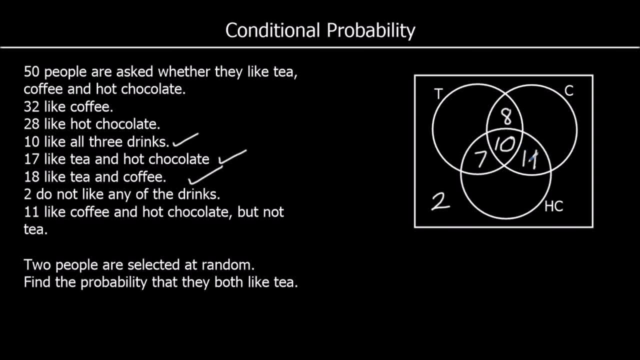 bit is coffee and hot chocolate, but not tea. So let's go back to the top 32, like coffee. so we've got 8 and 10, which is 18,, plus 11,, 20,, 30. So we've got 29,. we need 32,, so that's 3 more. 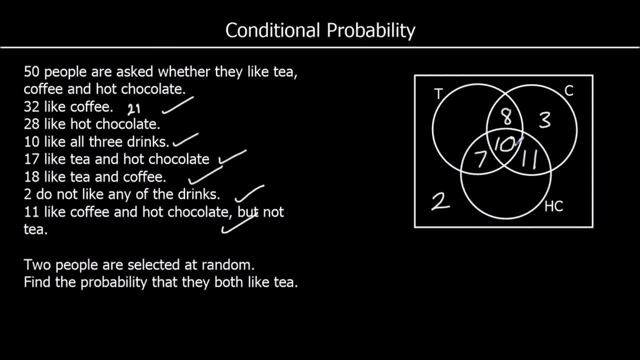 28 like hot chocolate. we've got 10, plus 7 is 17,, plus 11 is 28,. so that's all 28,. there's no one that just likes hot chocolate, and with the missing number they add up to. 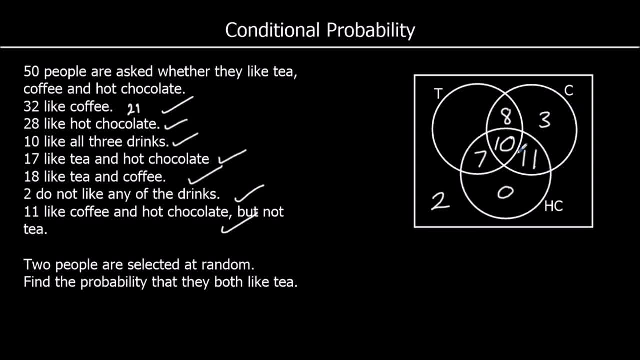 50. So the coffee circle was 32 people, So we've got 18, plus 7 is 17,, plus 11 is 28,. so that's all 28,. there's no one that just likes hot chocolate, and with the missing number they add up to 50. 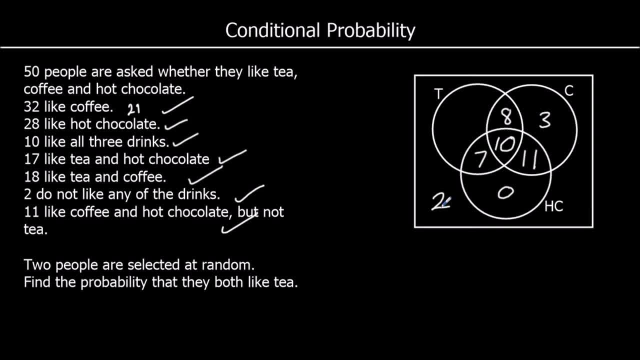 So we've got 18 plus 7 is 39, plus 2 is 41,, so 50 take away 41 is 9, so that must be 9.. So the question says 2 people are selected at random. find the probability they both. 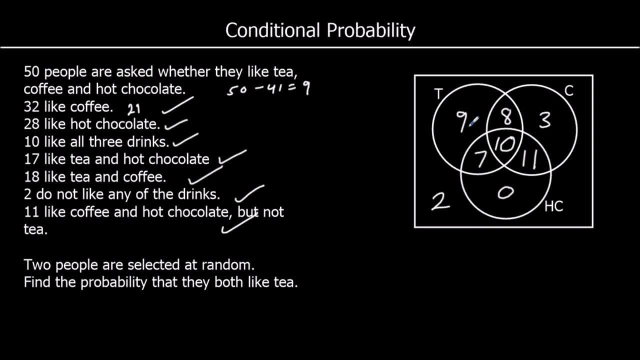 like tea. So how many people like tea? So the tea circle is 10 people: 10 plus 8, which is 18, plus 7, which is 25 plus 9, which is 34. so our T circle is 34 people. so 34. 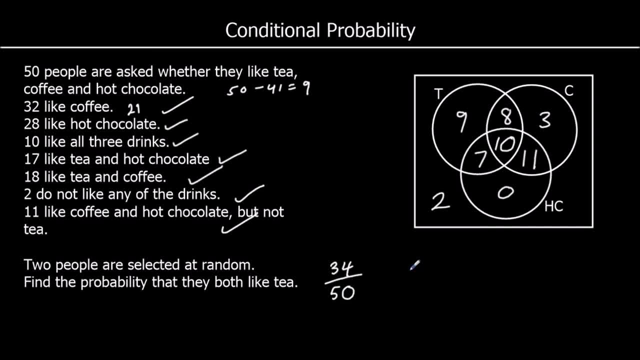 out of 50. 34 out of 50 like T. we're selecting two people at random. so if the first person likes T, the probability of the first person likes T is 34 out of 50. and then if we take them out- we've already asked them what's the probability- the next person likes T. so there's 33 T likers left.